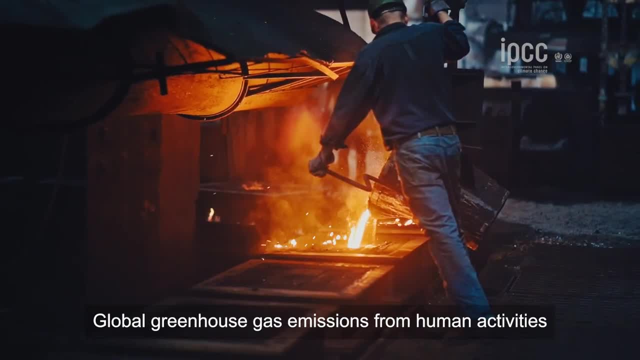 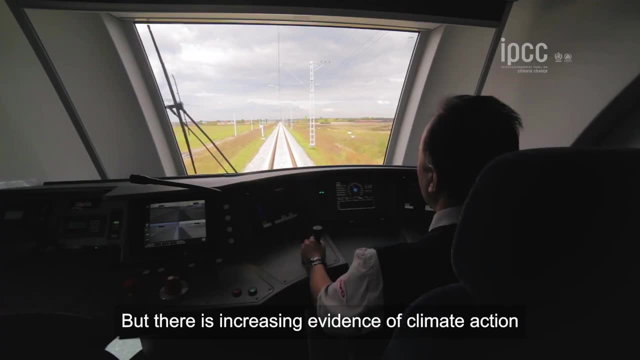 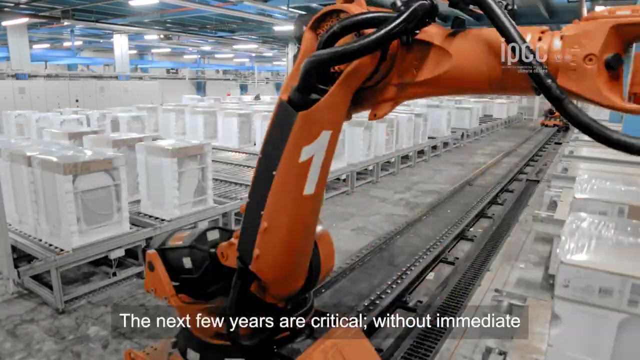 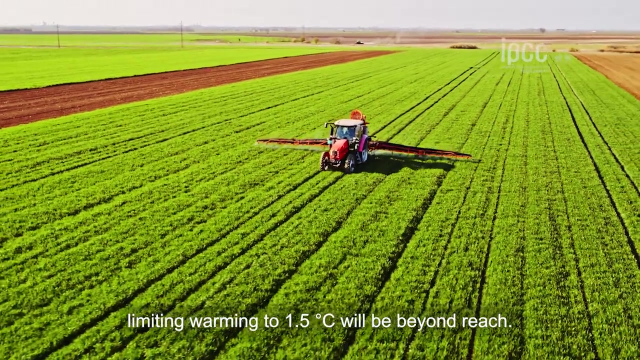 Global greenhouse gas emissions from human activities are at their highest levels in human history, But there is increasing evidence of climate action and the average annual rate of growth in global emissions has slowed in the last decade. The next few years are critical Without immediate and deep emissions reductions in all sectors, limiting warming to one and a. 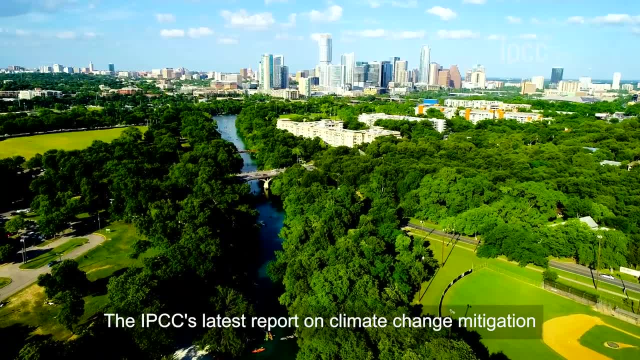 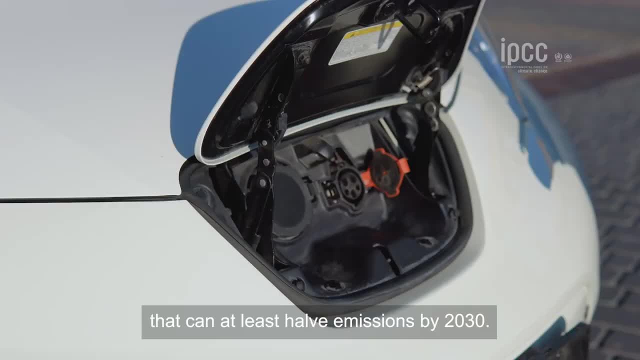 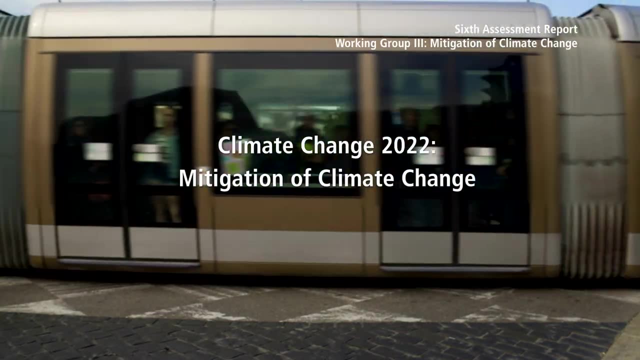 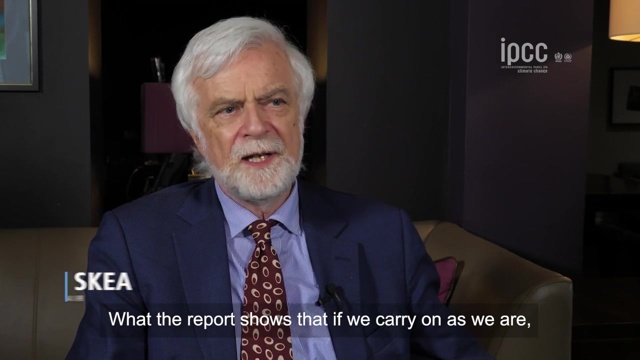 half degrees Celsius will be beyond reach. The IPCC's latest report on climate change mitigation shows that there are options available in every sector that can at least halve emissions by 2030.. What the report shows is that if we carry on as we are, we won't be able to limit global. 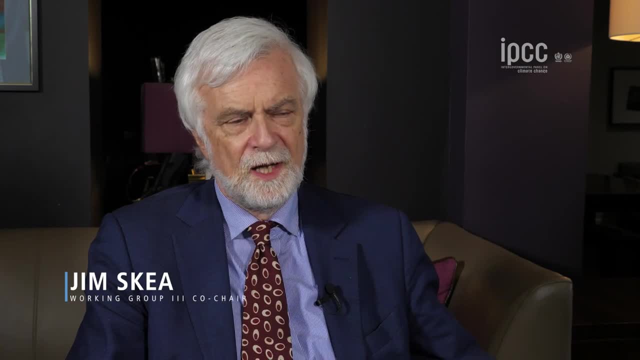 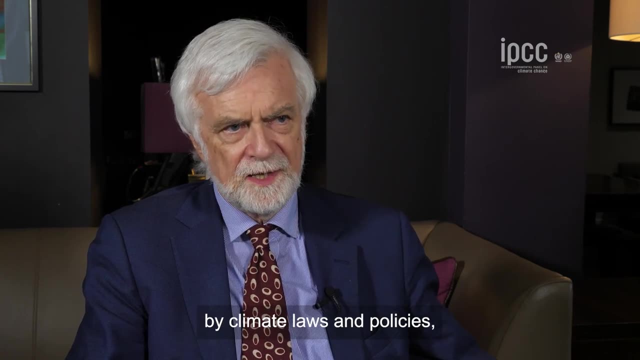 warming to two degrees. Never mind, We're only at 1.5. But we do find signs of progress. I mean, half the world's emissions are now covered by climate laws and policies And we're seeing the falling cost of renewable energy and big take-ups. 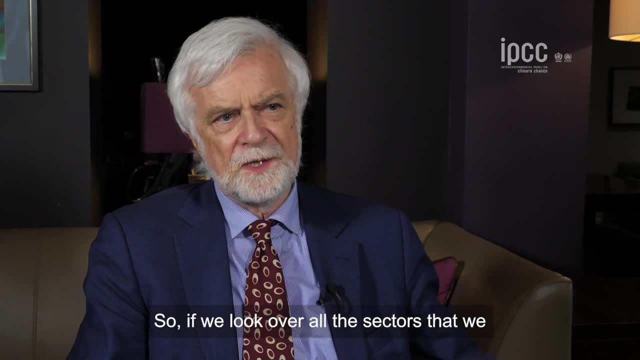 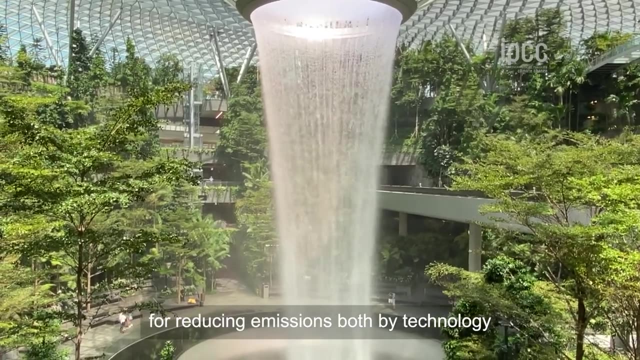 It is beginning to make a difference. So if we look over all the sectors that we cover in the report, we can find options everywhere for reducing emissions, both by technology and by behavioural change, And when you add it all up, you could see the capacity to cut emissions by a third. 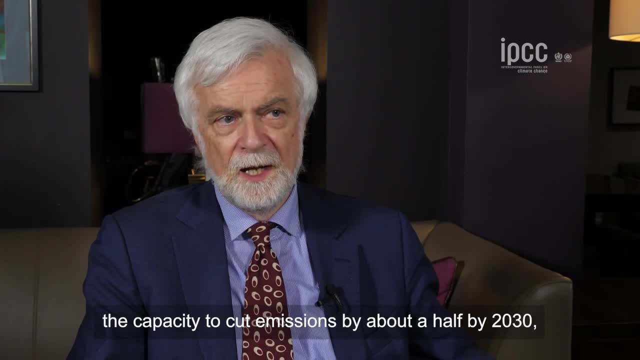 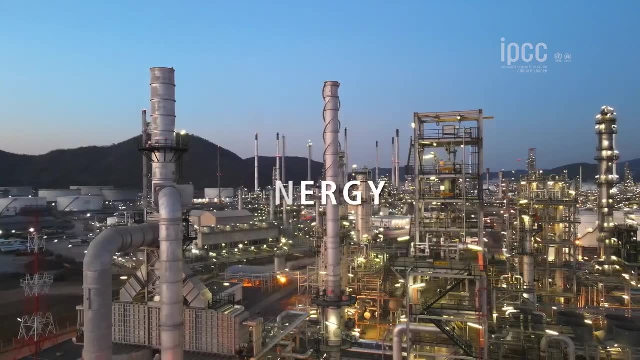 So we're now at 1.5.. So if we look over all the sectors that we cover in the report, we can see the capacity to cut emissions by about a half by 2030. But it would need very prompt and ambitious action for that to actually happen. 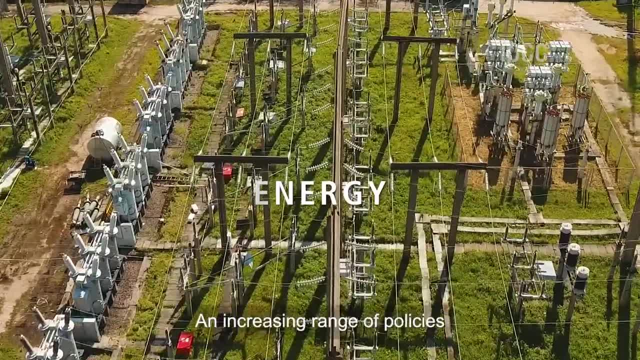 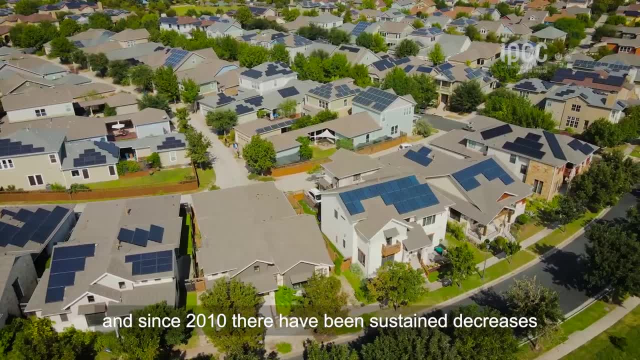 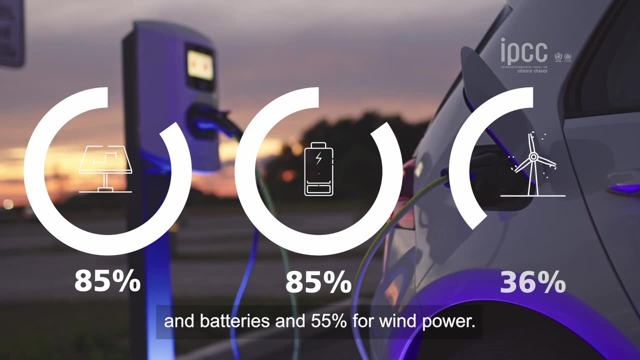 The energy sector accounts for about one-third of all emissions. An increasing range of policies and laws have enhanced energy efficiency And since 2010,, there have been sustained decreases in costs, with reductions of 85% for solar energy and batteries and 55% for wind power. 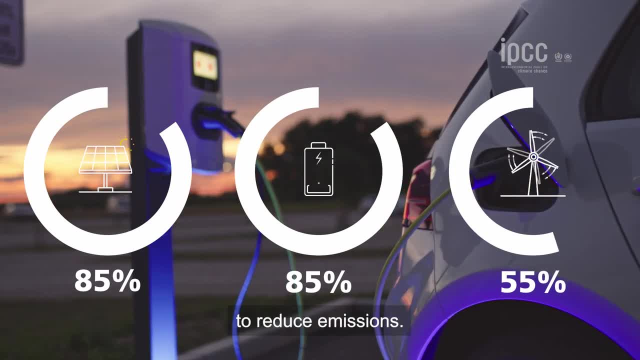 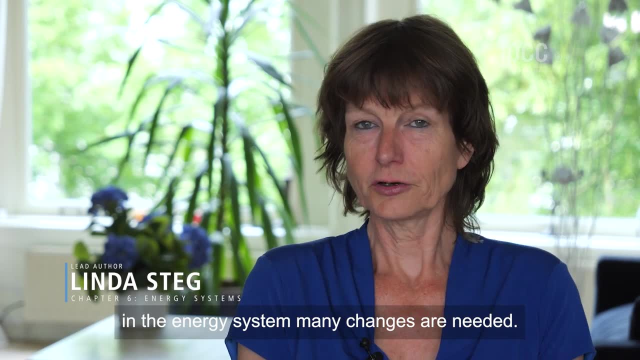 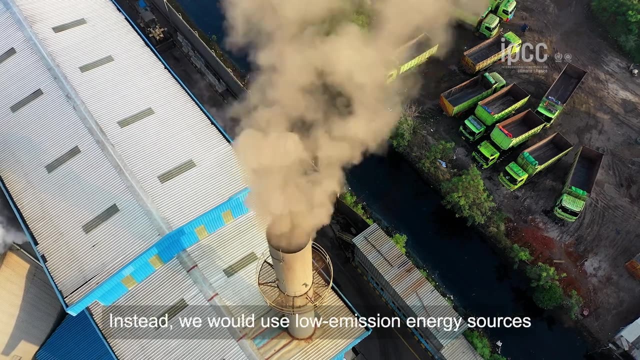 Major changes have been made. Solar transitions are required in this sector to reduce emissions. To reduce greenhouse gas emissions in the energy system. major changes are needed. We would use far less fossil fuel, meaning that fossil fuels remain in the world. Instead, we would use low-emission energy sources such as wind and solar and alternative. 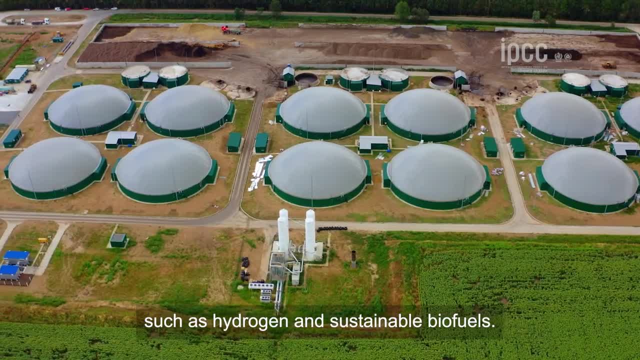 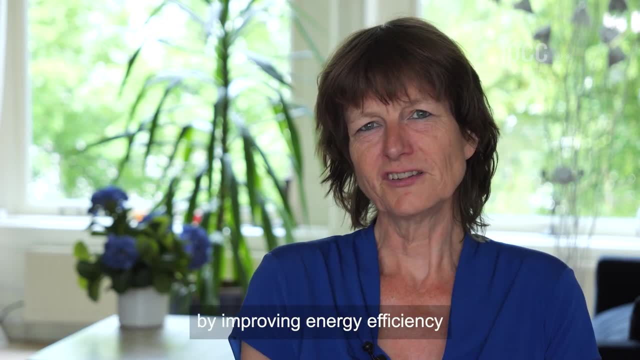 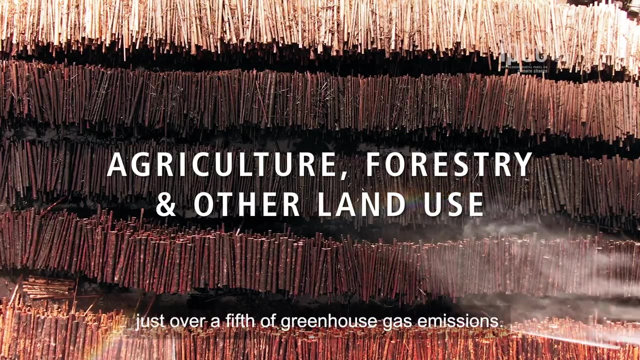 energy carriers such as hydrogen and sustainable biofuels. Moreover, we would use far less fossil fuels, meaning that fossil fuels will remain in the world use far less energy than today. by improving energy efficiency and promoting energy conservation, Agriculture, forestry and other land use contribute just over a fifth of greenhouse. 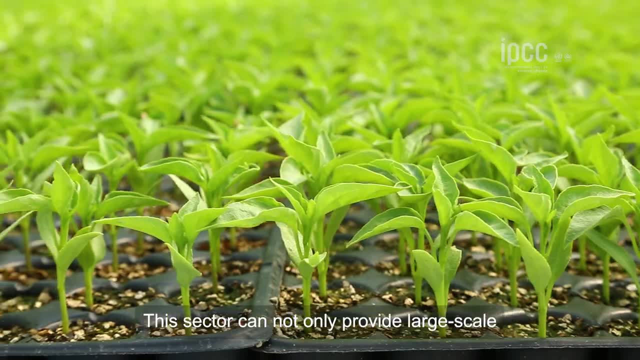 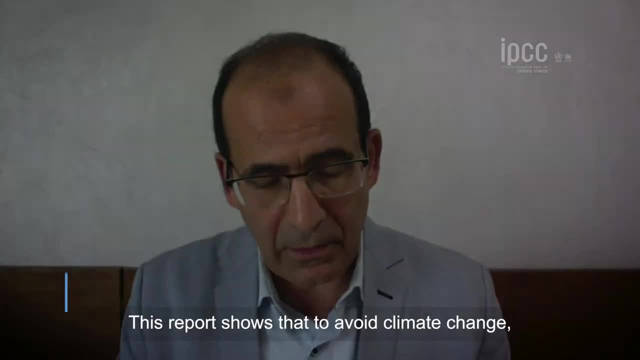 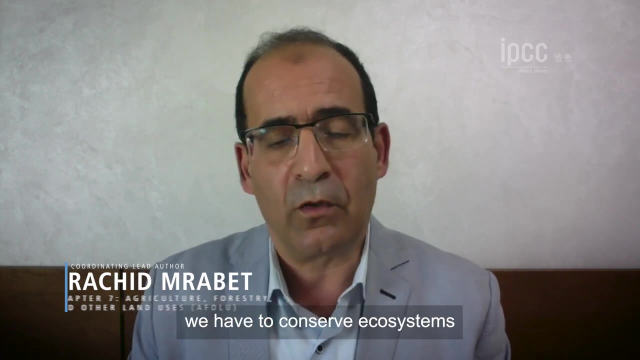 gas emissions. This sector can not only provide large-scale greenhouse gas emissions reductions, but can also remove and store carbon dioxide at scale. This report shows that to avoid climate change, we have to conserve ecosystems and improve food systems. We have to restore 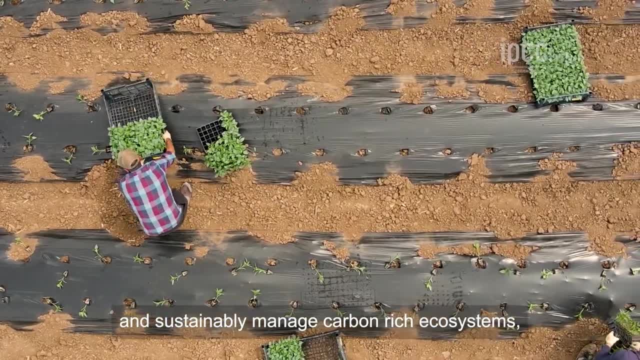 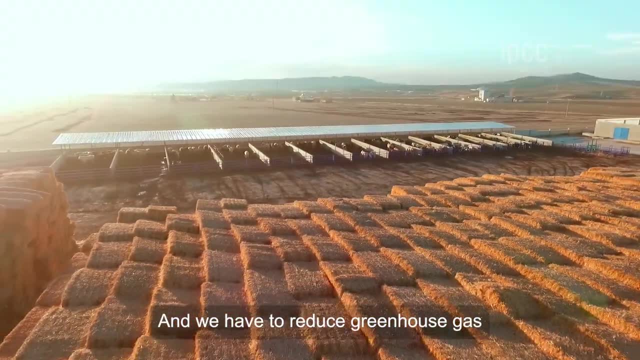 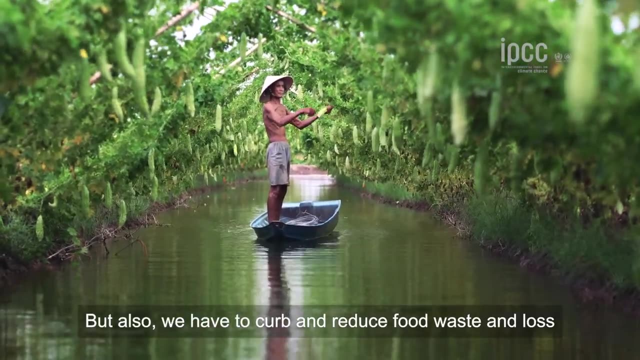 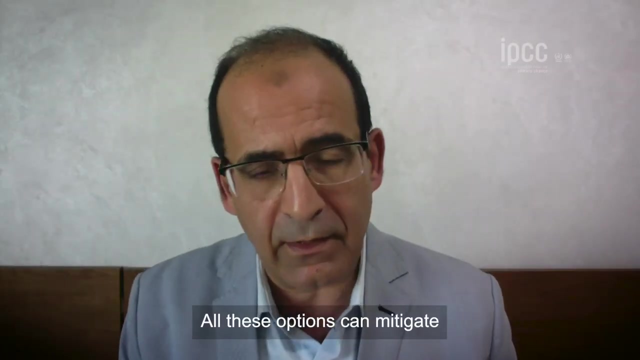 protect and sustainably manage carbon-rich ecosystems like forests and grassland, and we have to reduce greenhouse gas intensity of food production systems. But also we have to curb and reduce food waste and loss and shift more sustainable and healthy diets. All these options can mitigate 8 to 14 gigatons of CO2 per. 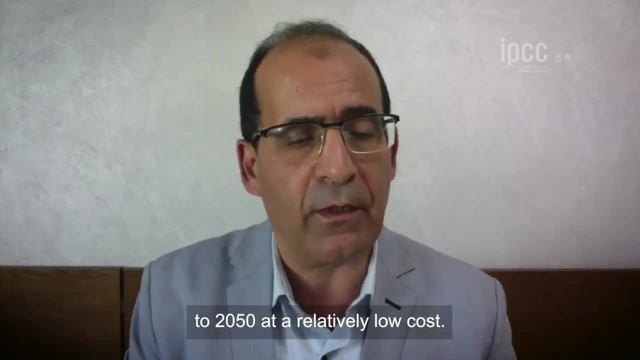 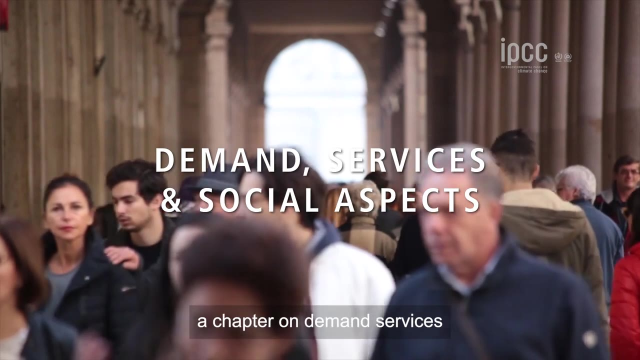 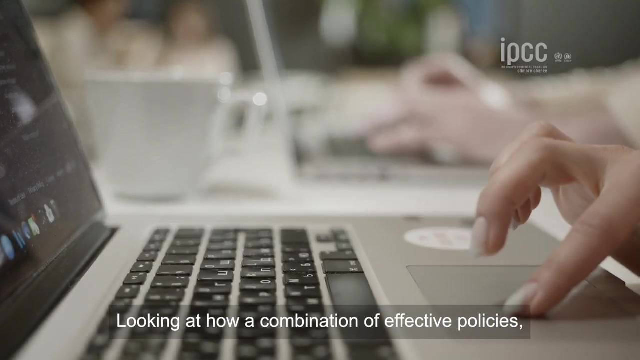 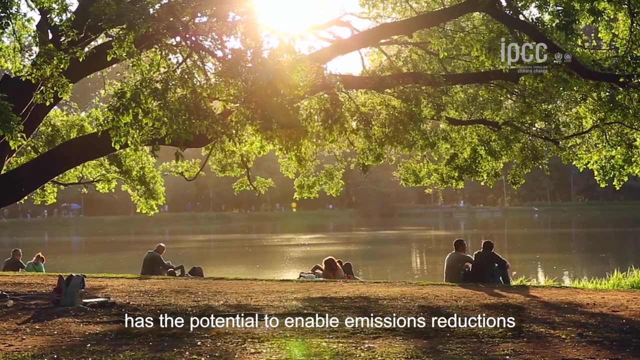 year, from now up to 2050, at relatively low cost. This is the first IPCC assessment to include a chapter on demand services and social aspects of mitigation, looking at how a combination of effective policies, improved infrastructure and technologies leading to behavioral change has the potential to enable emissions reductions. 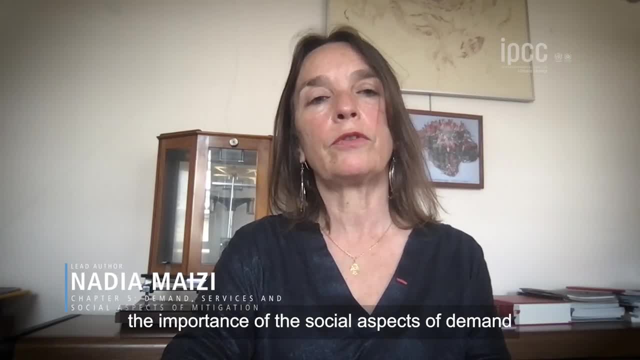 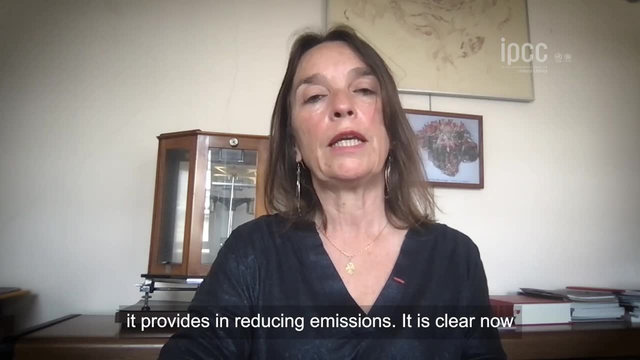 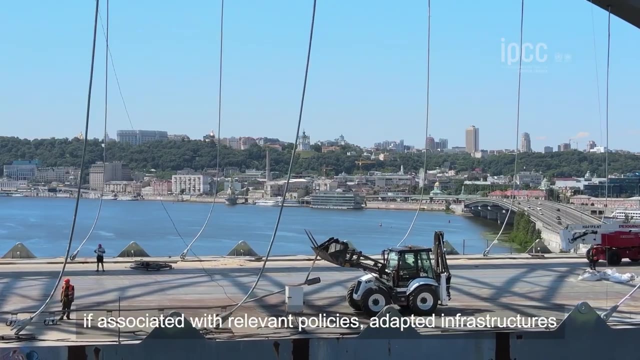 This report shows for the first time the importance of the social aspects of demand and the huge potential it provides in reducing emissions. It is clear now that human behavior is the center of the problem and also the solution, if associated with relevant policies, adapted infrastructures and if technologies are. 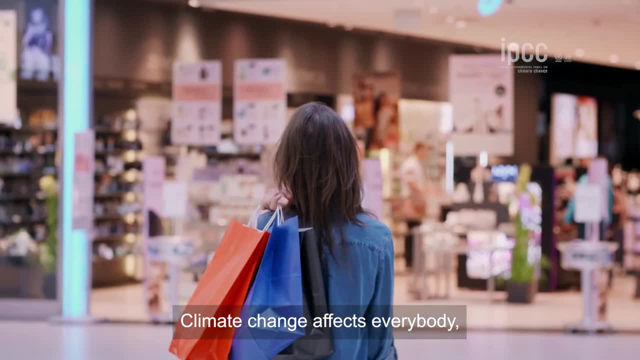 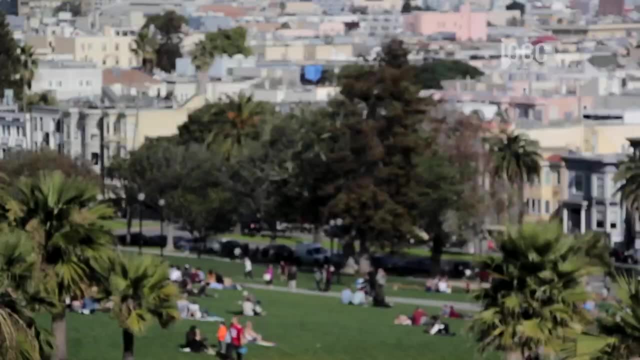 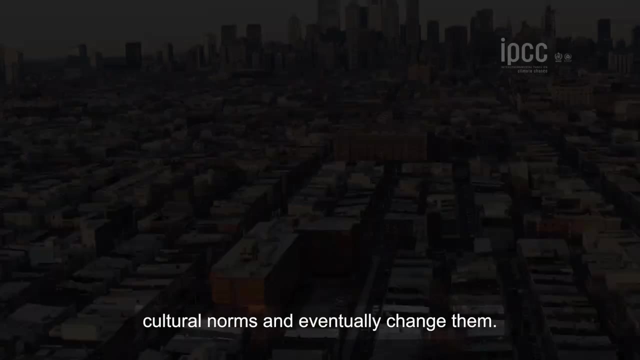 available. Climate change affects everybody, but 10% of the richest people are responsible for 40% of the emissions, So they need to question the lifestyles, cultural norms and eventually change them. Cities and other urban areas, where most of the world's population lives, are responsible for. 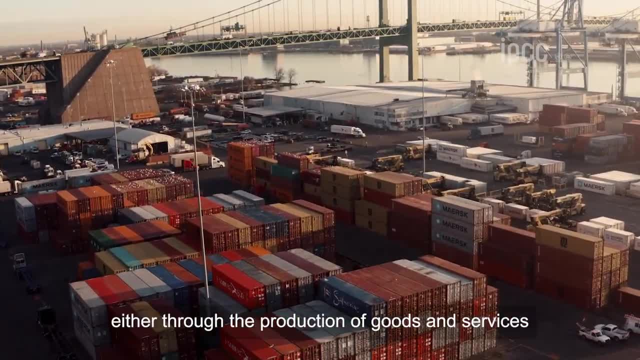 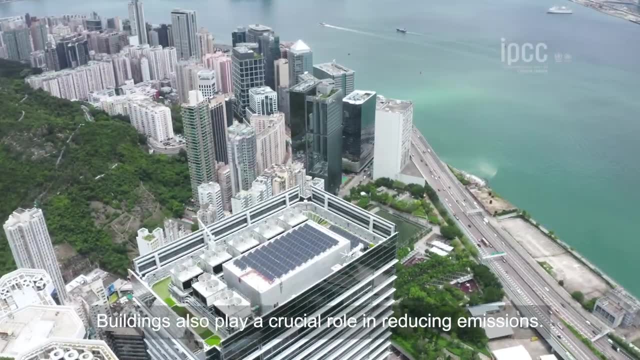 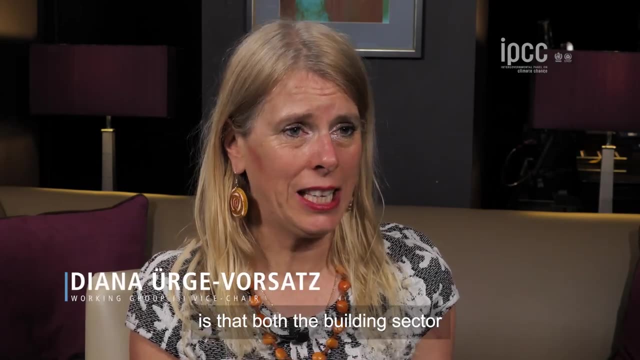 more than two-thirds of global greenhouse gas emissions, either through the production of goods or those that are transported to cities. Buildings also play a crucial role in reducing emissions. What this assessment shows is that both the building sector and cities can go to net zero. 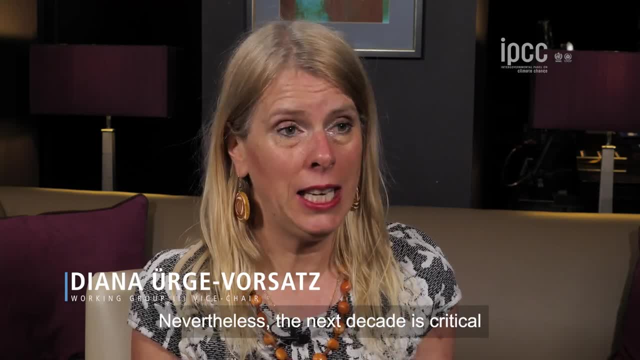 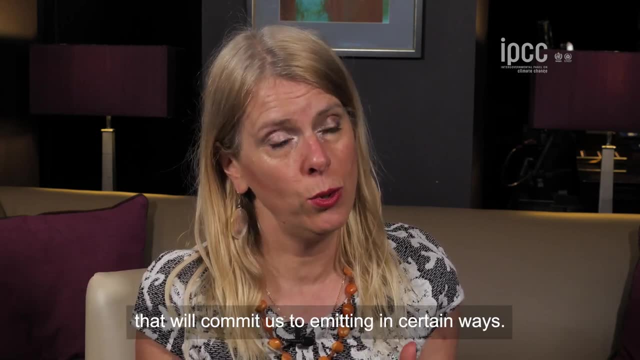 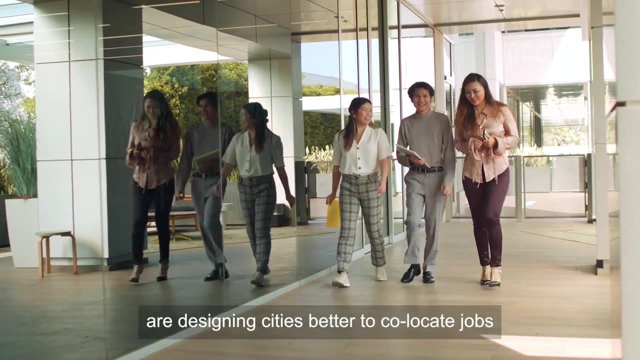 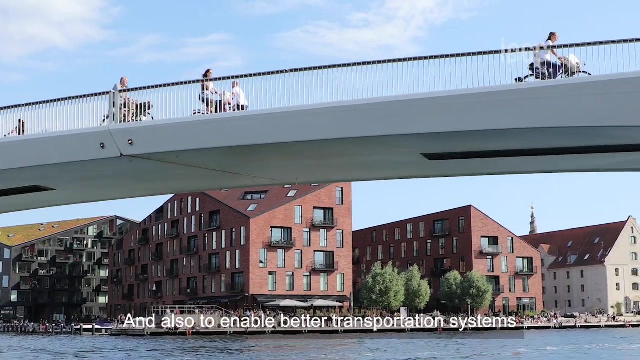 carbon dioxide emissions towards the middle of the century. Nevertheless, the next decade is critical because both of these involve infrastructure that will commit us to emitting in certain ways In cities. the most important areas of action, like the cities themselves, are designing cities better to co-locate jobs and homes together, and 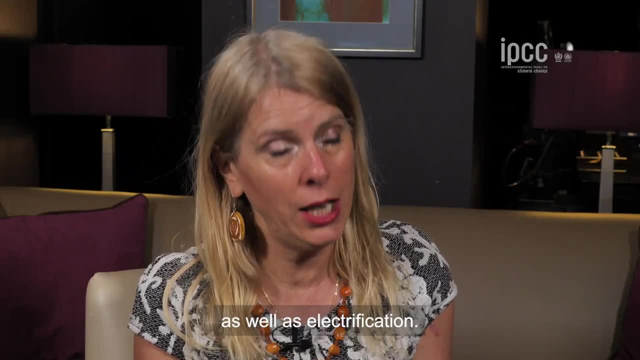 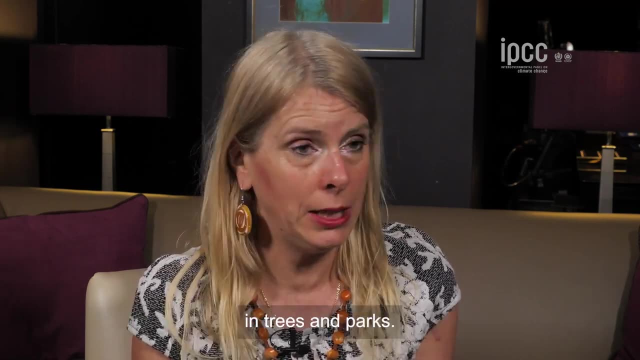 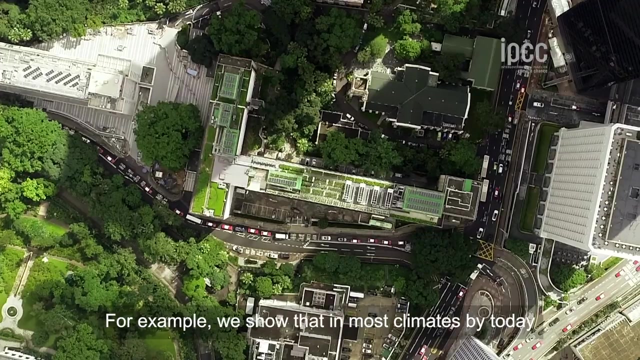 also to enable better transportation systems, where we actually can perhaps do active transport As well as electrification. And finally, removing or storing carbon dioxide in the urban environment, for example in trees and parks. Buildings can also help, for example. we show that in most climate. 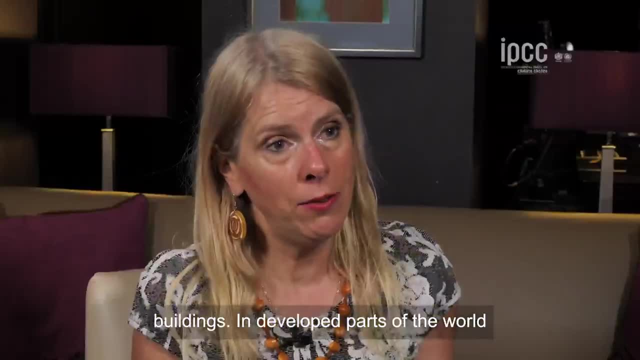 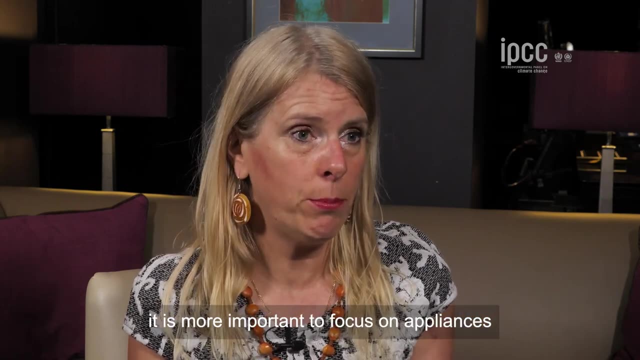 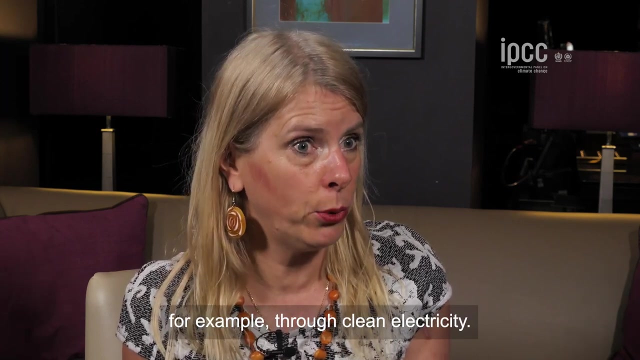 net zero energy and net zero carbon buildings. In developed part of the world, retrofit is more important, whereas in developing countries it is more important to focus on appliances and supplying the energy in clean ways, for example, through clean electricity, The ways that we use transport. 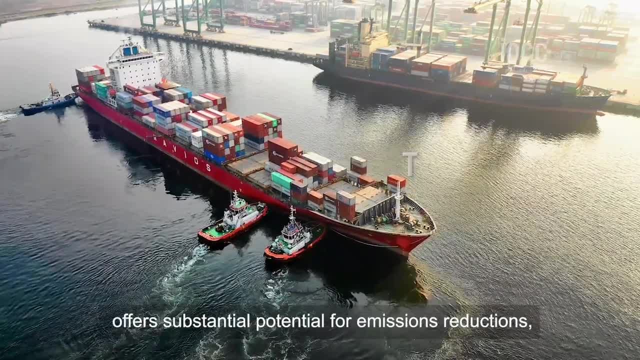 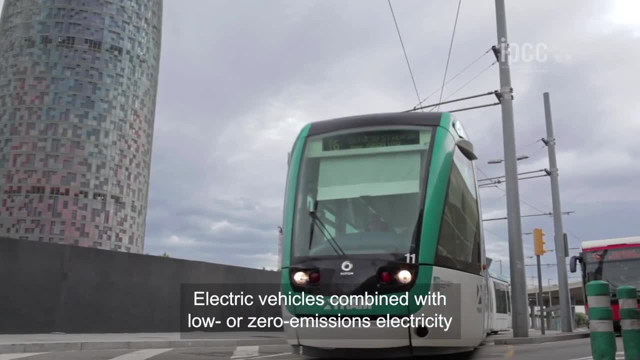 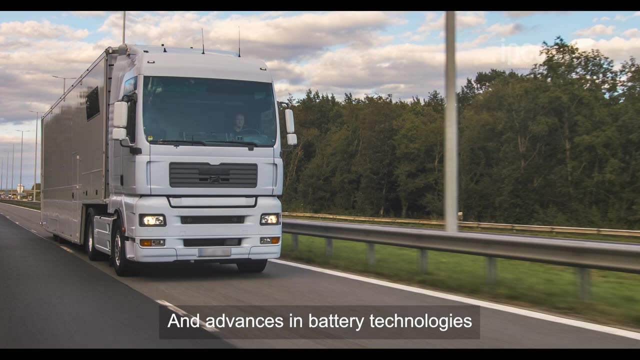 whether for travel or to transport goods, offers substantial potential for emissions reductions, But this depends on decarbonizing the power sector. Electric vehicles combined with low or zero emissions electricity offer the greatest potential, and advances in battery technologies could assist in the electrification of trucks. 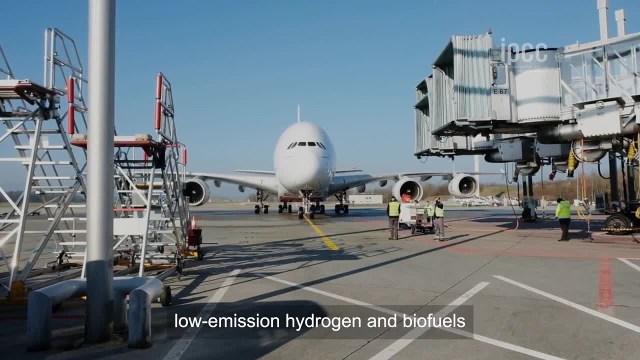 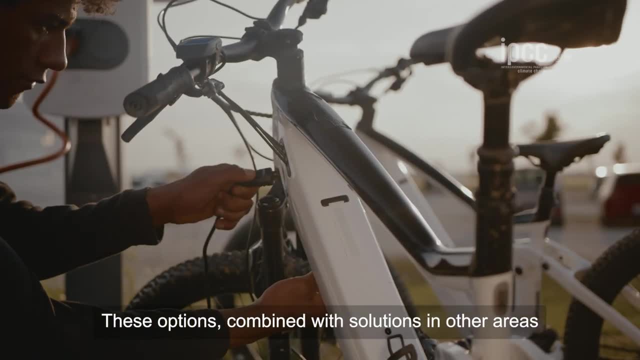 For shipping and aviation, which are harder to decarbonize. low-emission hydrogen and biofuels offer alternatives to going electric. These options, combined with solutions in other areas like cities and reducing demand, offer us a way forward in the transport sector. 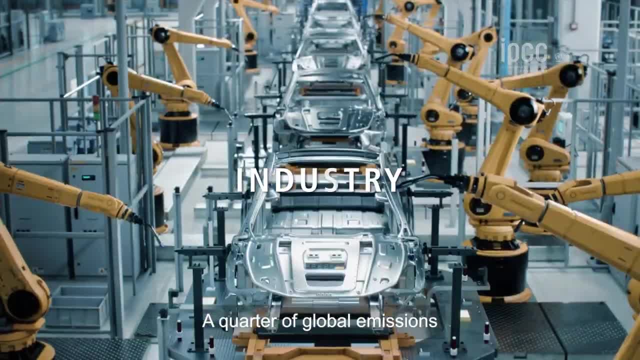 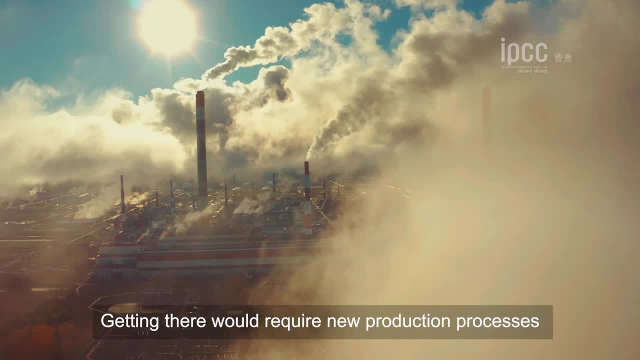 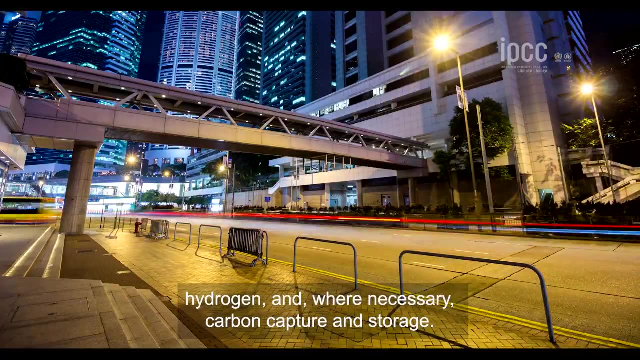 A quarter of global emissions comes from the industry sector, where achieving net zero is challenging. Getting there would require new production processes and using low and zero greenhouse gas, electricity, hydrogen and, where necessary, carbon capture and storage. The industrial sector has increased rapidly. 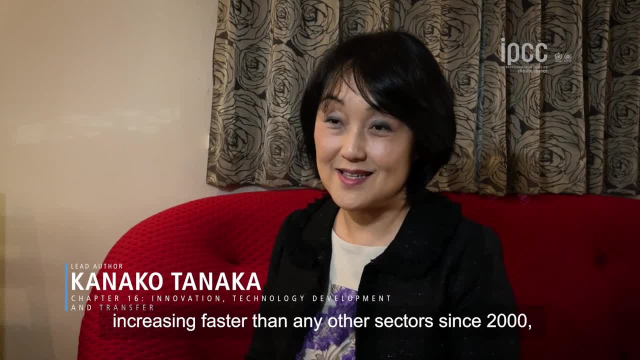 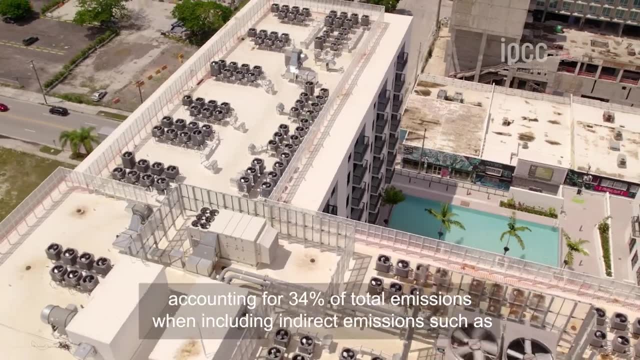 from the emissions of any other sector since 2000,. and the efficiency of the industry has increased rapidly. and the efficiency of the industry has increased rapidly. thus, the total emissions from the production of hydrogen can be estimated at 34% of the total emissions. 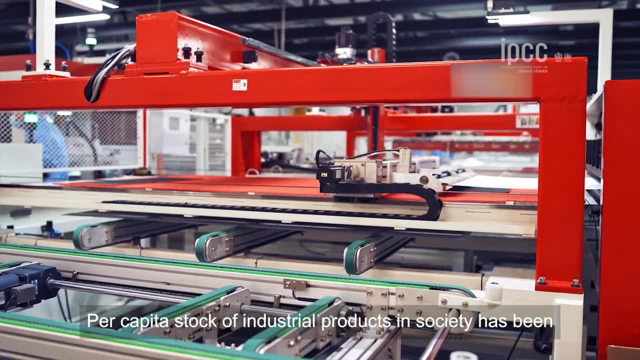 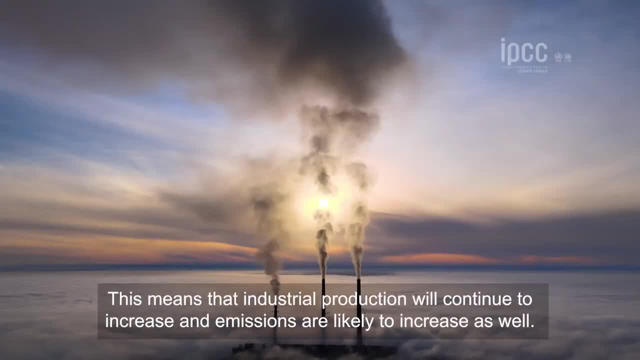 In the world's leading countries, the number of products used by the society has become the number one priority, but it's growing worldwide. The number of industrial produce can increase, with the possibility of the emissions increasing. How can we reduce this amount of emissions? 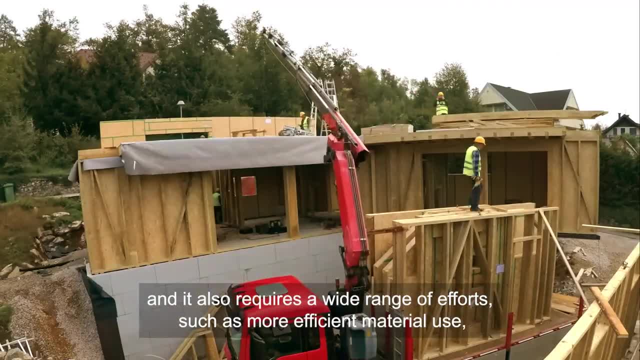 Low-emission hydrogen and biofuels are still very important and efficient use of materials, use of products and low emissions energy efficiency are key and efficiency of the industry are still very important and efficient use of materials, use of products and low emissions energy efficiency are key. 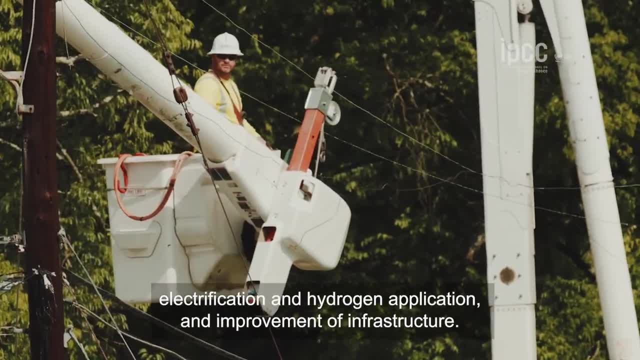 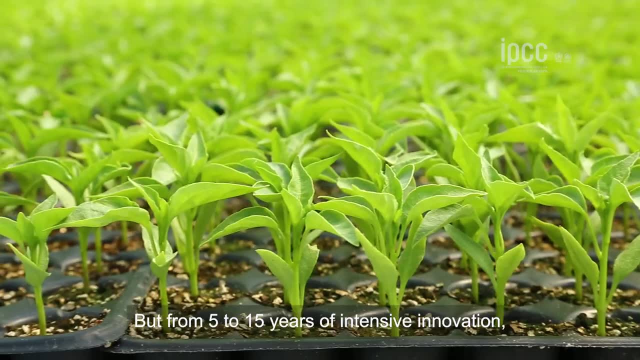 and recycling, as well as the use of electricity and hydrogen, as well as the maintenance of the infrastructure and so on. There is certainly technology to make zero emissions, but we need to focus on technological innovation, commercialization and new industrial development in the next 5 to 15 years. 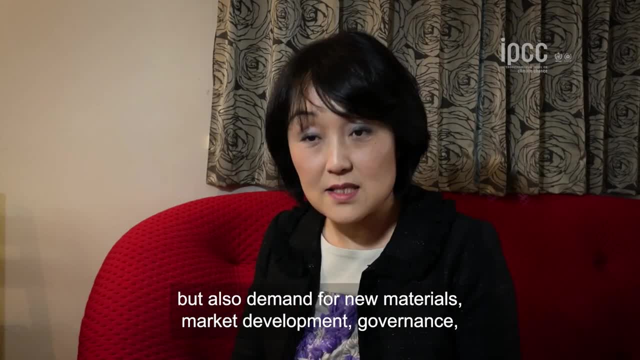 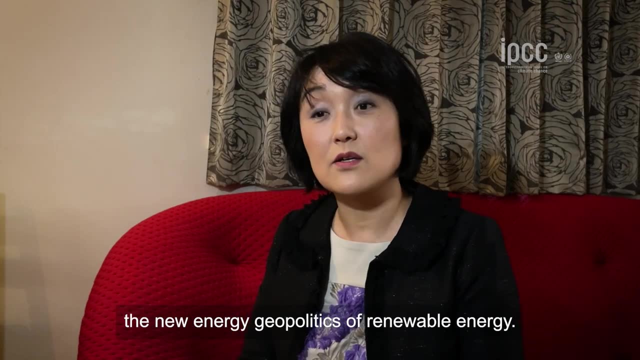 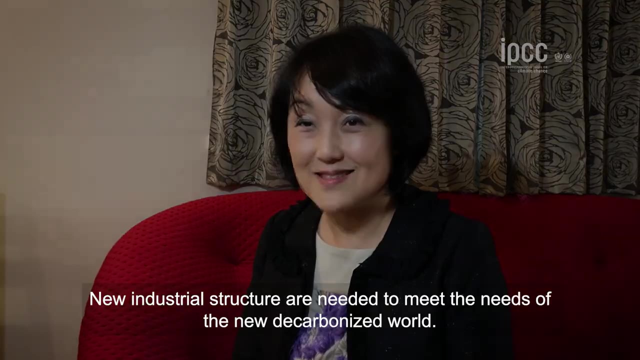 Not only technology development, but also the demand for new materials for the new society, the development of the market governance and the new value chain from the new energy economy called Cyanide. It is necessary to build a new industry that suits the new world. 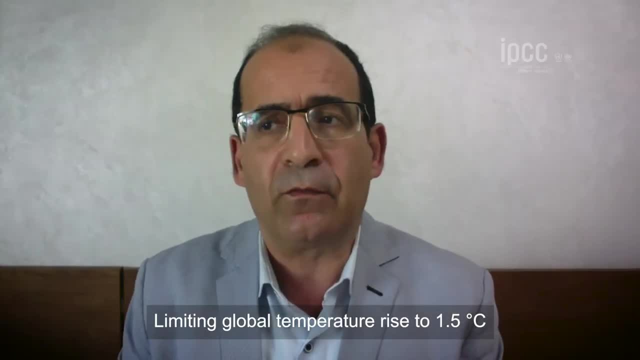 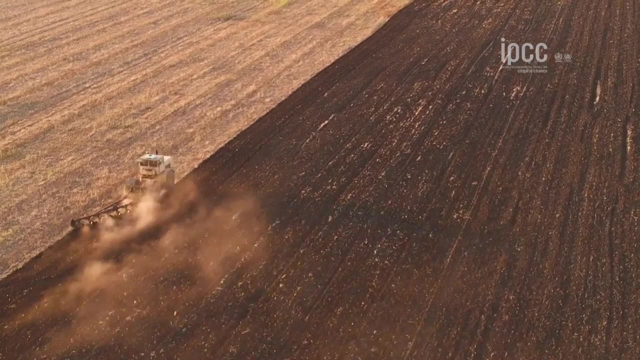 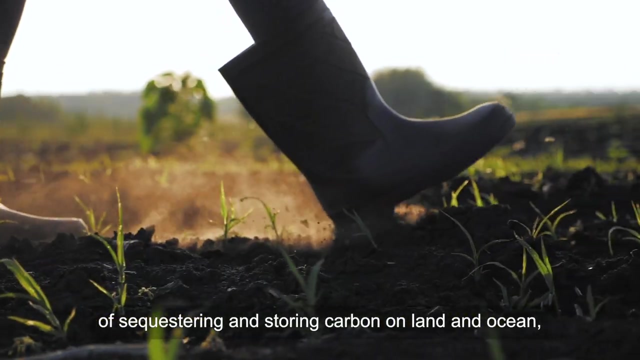 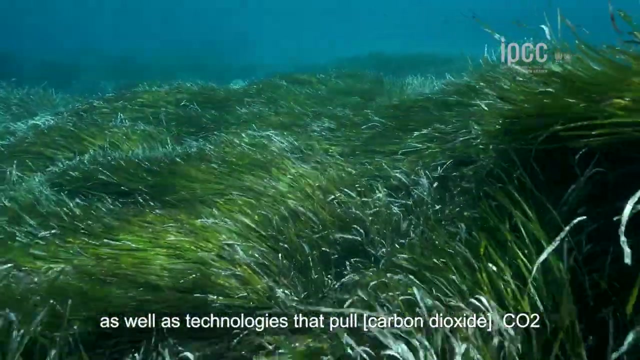 Limiting global temperature rise to 1.5 °C will not be possible without carbon dioxide removal. Carbon dioxide removal approach can be either natural solution, as sequestering and storing carbon on land and ocean, as well as technologies that pool. carbon dioxide removal approaches can be either natural solution, as sequestering and storing carbon on land and ocean, as well as technologies that pool. 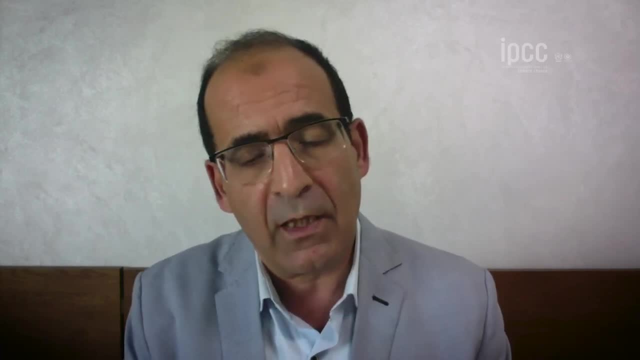 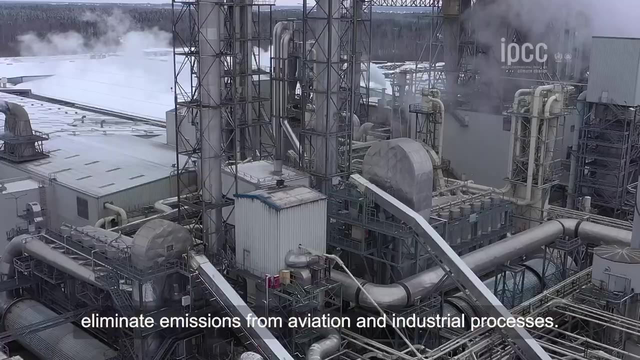 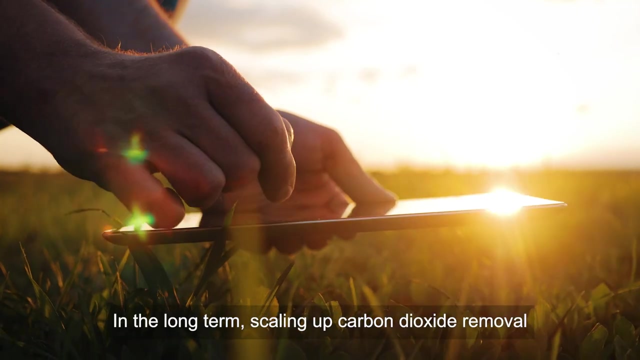 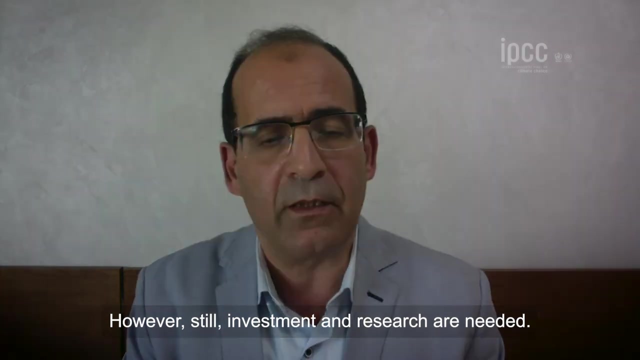 CO2 directly out of the atmosphere. Carbon dioxide removal can counterbalance how to eliminate emission from aviation and industrial processes. in the long term, Scaling up carbon dioxide removal could reverse global warming. However, still investment and research are needed. The next few years will be critical. 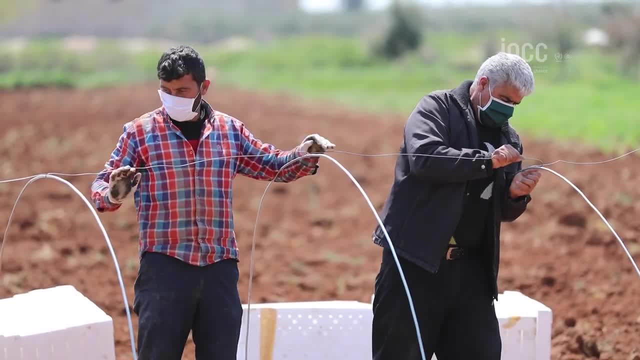 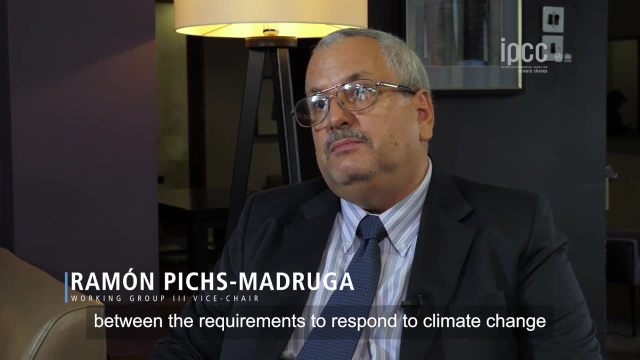 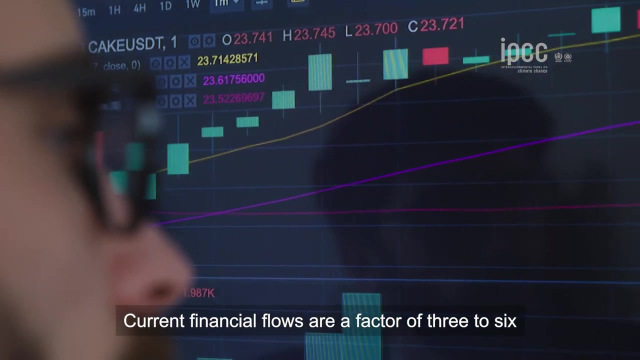 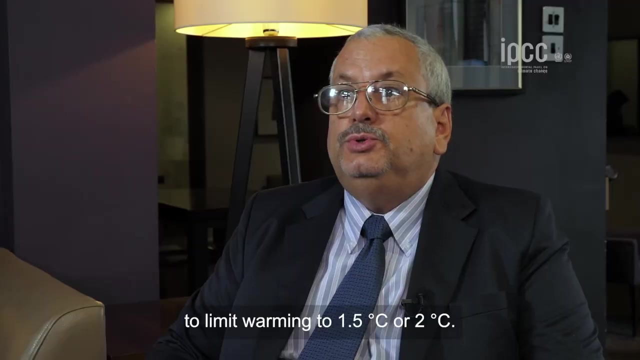 but there are ways to improve our chances of success. With regard to finance, there is a considerable gap between the requirements to respond to climate change and the existing financial flows. Current financial flows are a factor of three to six lower than the requirements by the year 2030. 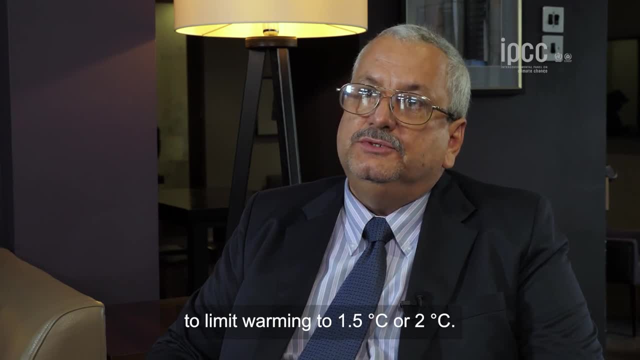 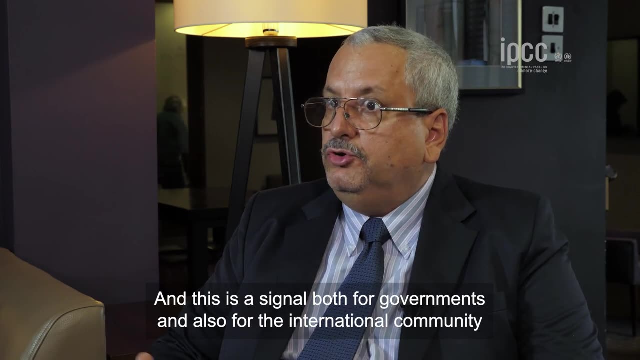 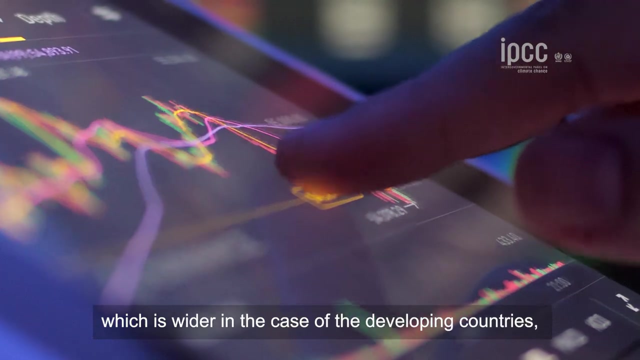 to limit warming to 1.5 degrees Celsius, or two degrees. This is a signal both for governments and also for the international community with regard to the need to close this gap, which is wider in the case of the developing countries, taking into account the limited capacity they have. 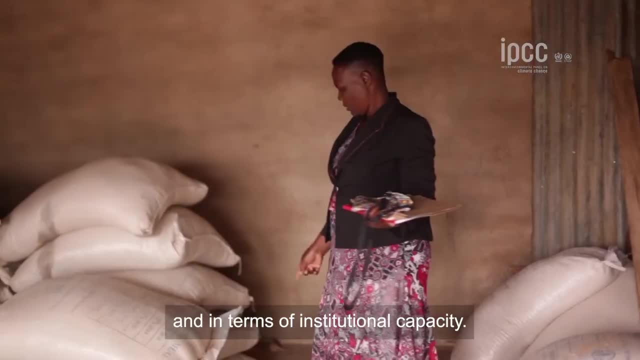 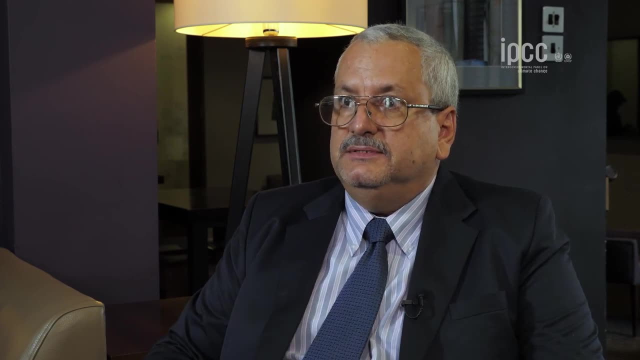 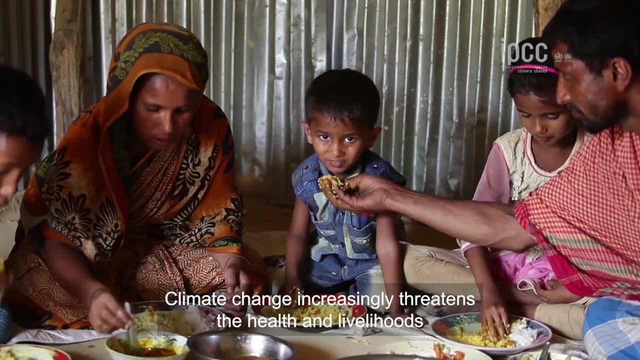 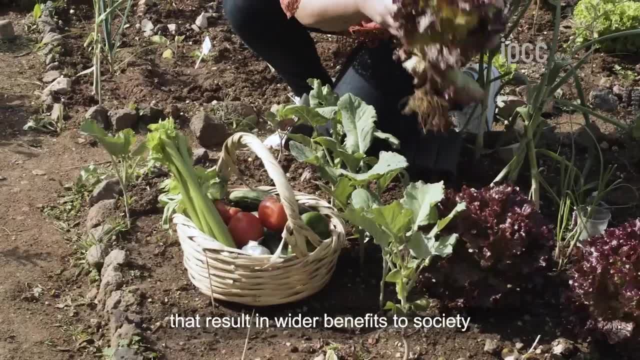 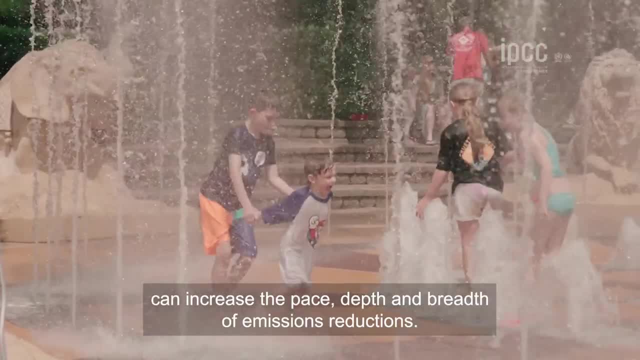 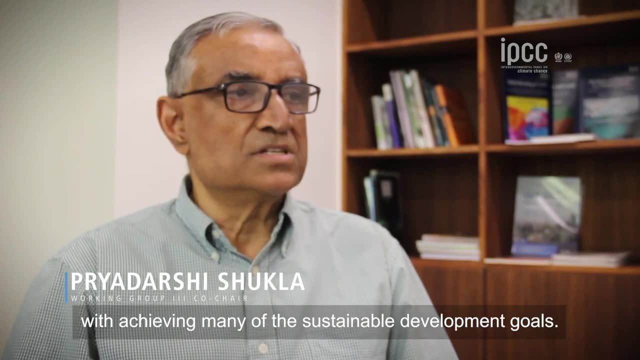 In all countries. actions to limit global warming that result in wider benefits to society can increase the pace, depth and breadth of emissions reductions. In this report we show how mitigation goes hand in hand with achieving many of the sustainable development goals. For example, if we look at the Sustainable Development Goals, 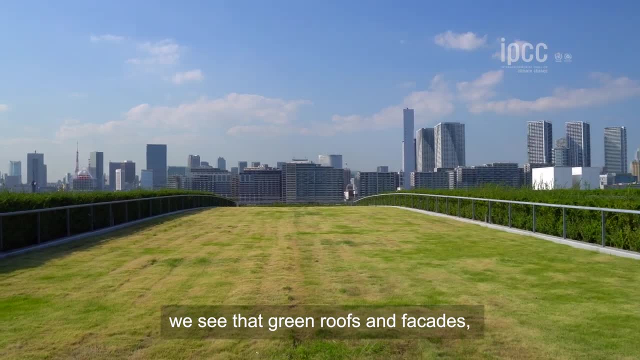 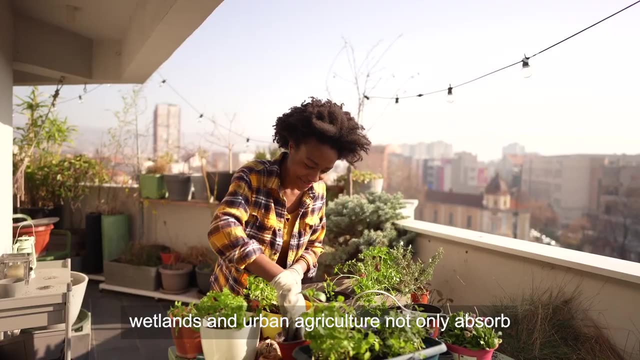 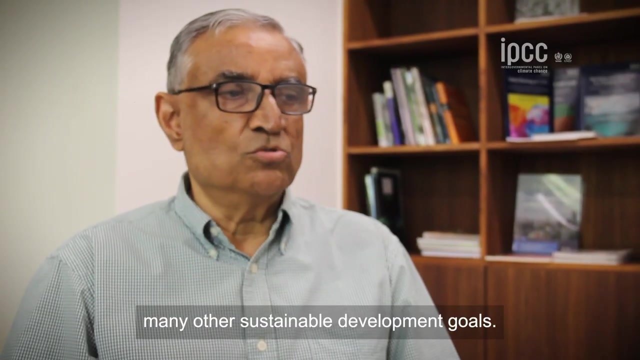 green and blue infrastructure. we see that green roofs and facades, networks of parks and open spaces, wetlands and urban agriculture not only absorb and store carbon but at the same time achieve many other sustainable development goals. They can reduce pressure on urban sewer systems. 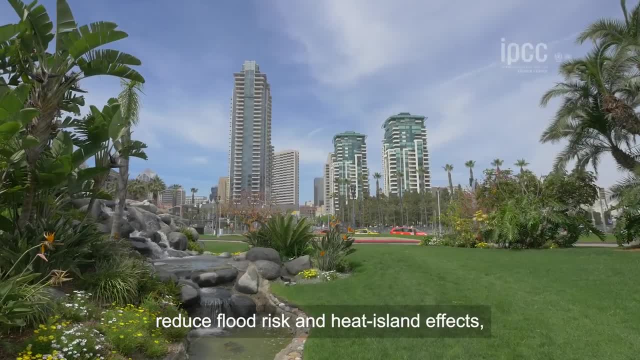 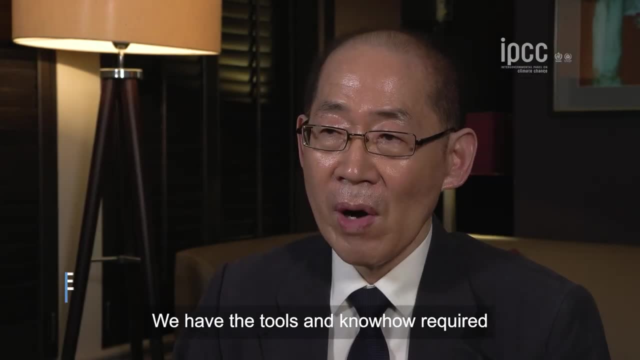